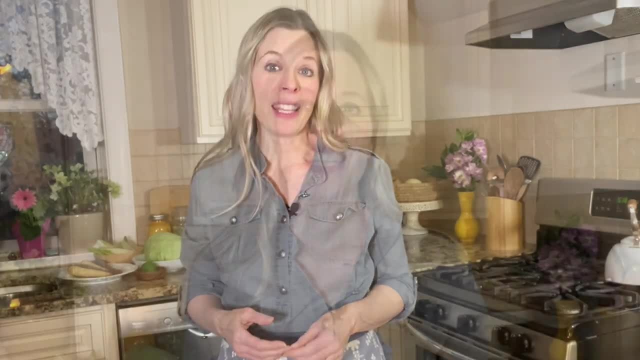 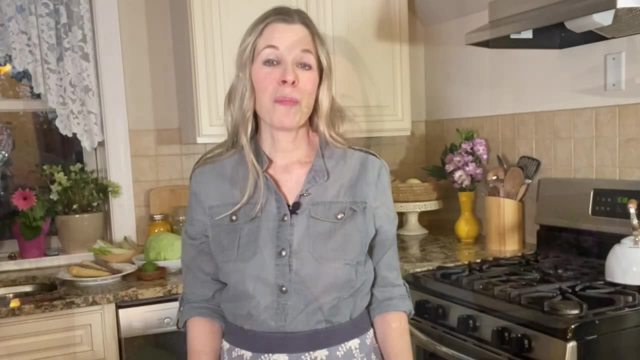 sit at a table rather than standing. We often do this for baking. If your child's hair is long, putting it up in a ponytail or a little bun will keep it out of the way, for both safety and hygiene. Prep side note, of course, we're also going to wash our hands before cooking as well. 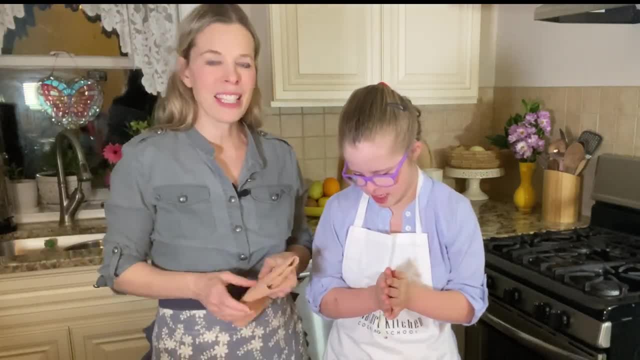 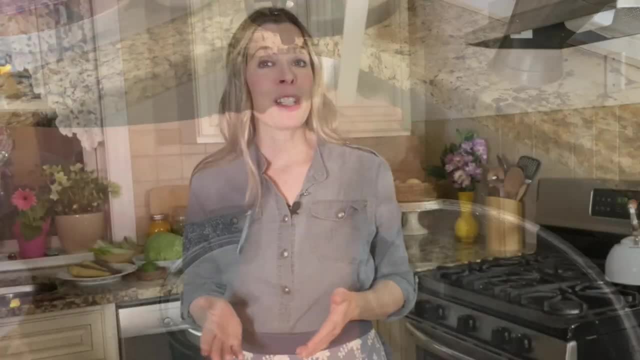 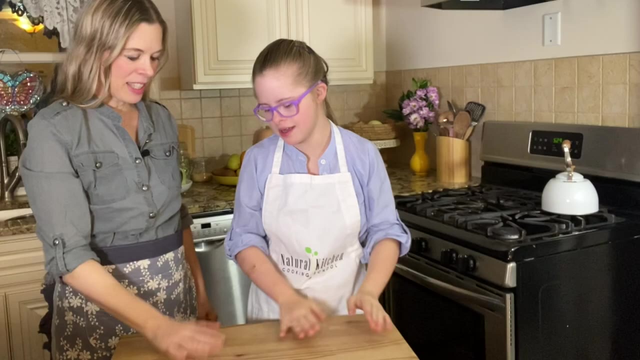 You want to wash your hands, You're gonna wash your hands. Yeah, Wash your hands. Tip number two: set up an organized prep area. If your child is standing, make sure that the counter is the right height for them. Let's see if this is a good height for you, right? We've cooked. 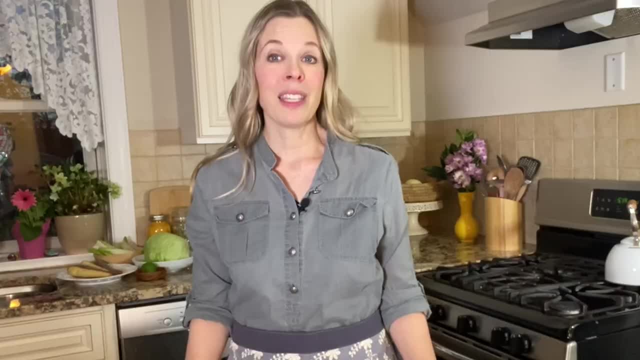 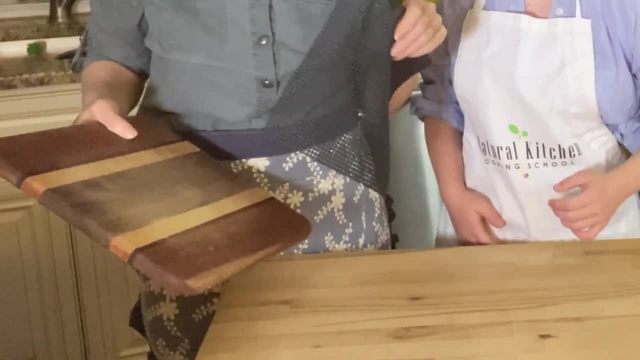 here before. this is a pretty good height for you, Using a stable stepstool if needed. For our cutting surface, I like to use a wooden cutting board And I put a piece of shelf liner beneath it to keep it stable. Put that right in the middle. 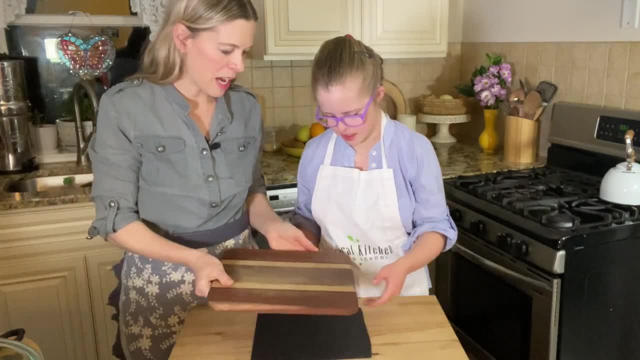 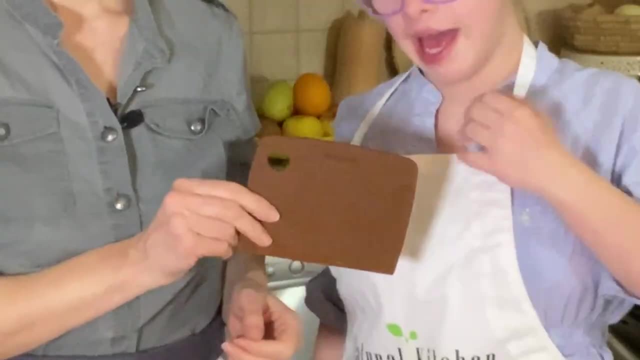 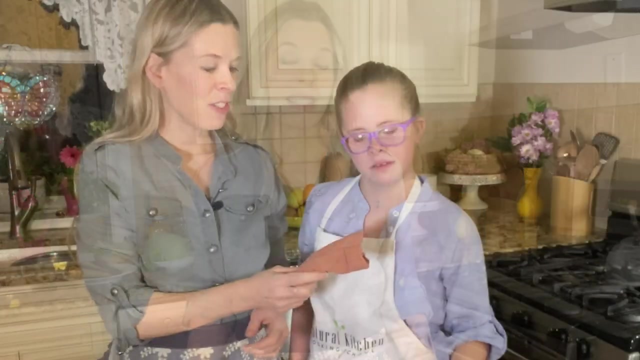 there. Yeah, then you can put your board on top. Having a container nearby for food scraps is helpful as well. Board scrapers make it easy to scoop up chopped ingredients, and a small damp towel often comes in handy to wipe down your board or clean up small spills. Here's our little damp towel. 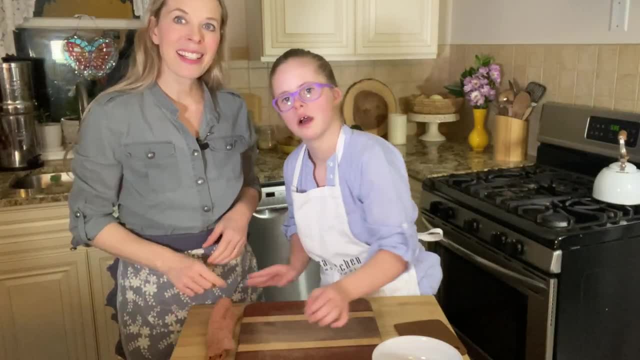 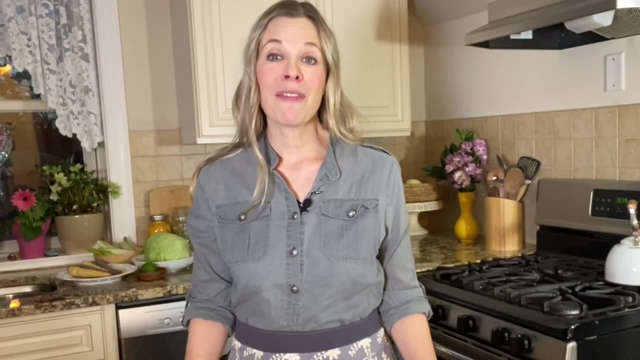 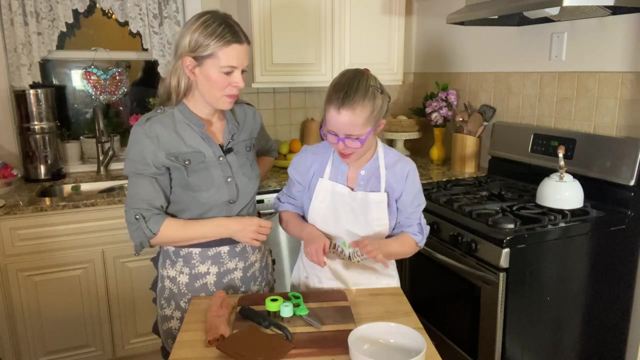 We'll keep that here. You look so cute in your little apron. Tip number three: select the right tools. Some of my favorites include kid safe knives. So here's your kid safe knife, right? Yep, this is good for cutting, And you can see that it's sharp enough to cut. 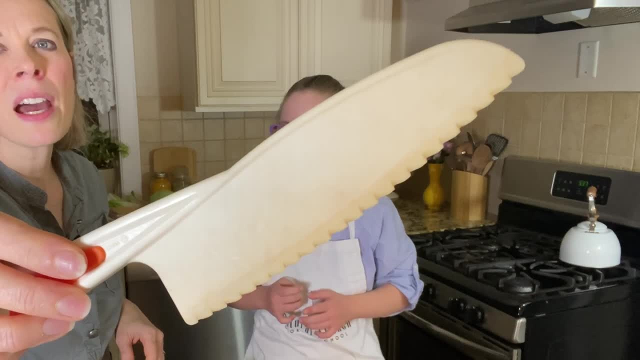 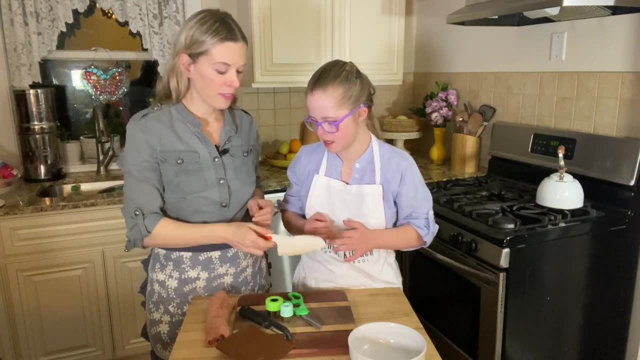 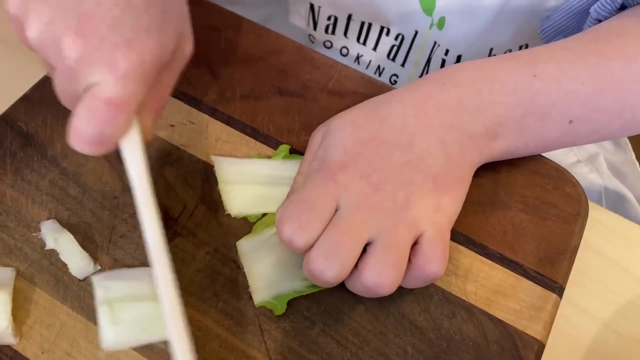 through softer vegetables, but it's not going to be sharp enough to cut your skin. I mean, yes, you could scratch yourself with it, but it's pretty kid safe. Alright, you like your little knife? Yeah, Yeah, Kitchen scissors. 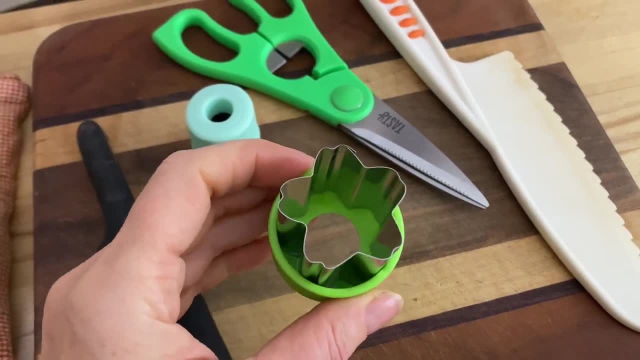 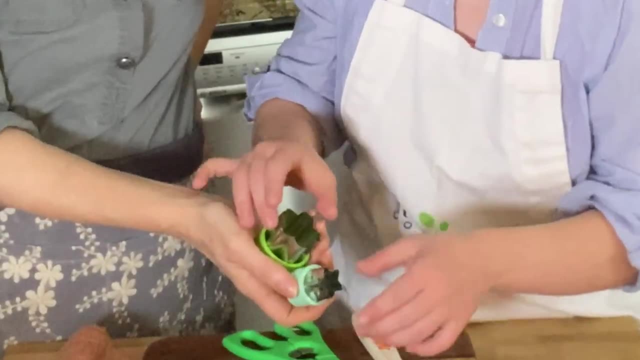 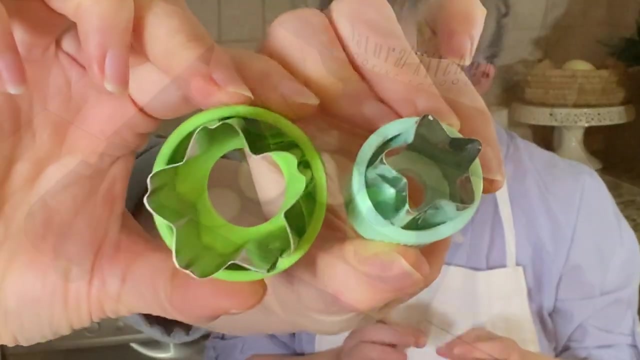 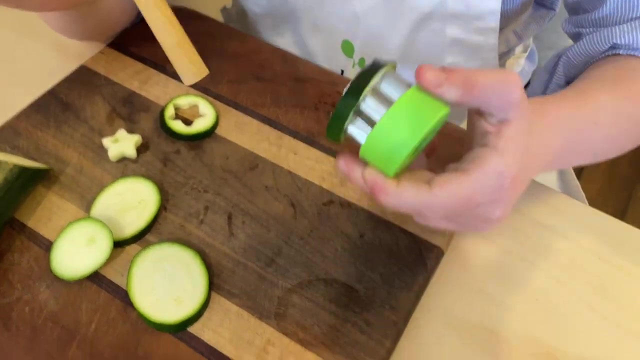 These adorable little cutters which make pretty flowers out of slices of cucumbers, carrots, zucchinis, apples and radishes. Little flower cutters. There it is. There it is, Yeah, Poke it out. Okay, put it out. 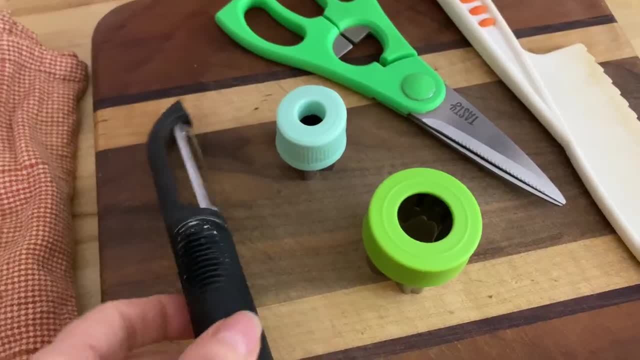 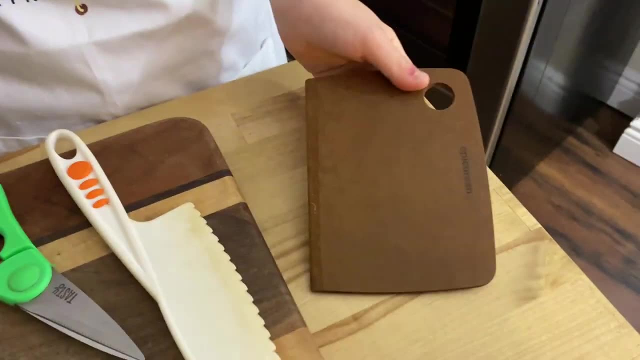 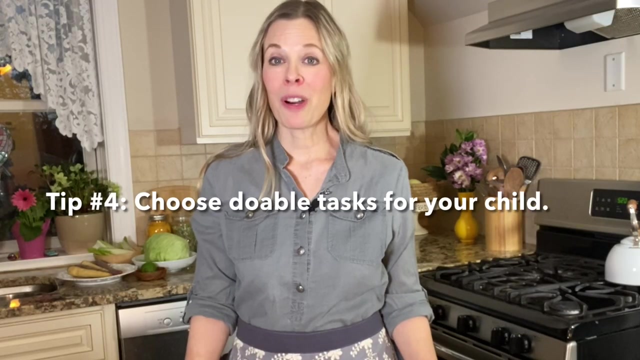 There it is. There it is, Yeah: Vegetable peeler And a pastry scraper. I like this one, since it doesn't have the sharp edges that a stainless steel scraper has. Tip number four: choose tasks that are doable for your child. Examples of skills that are: 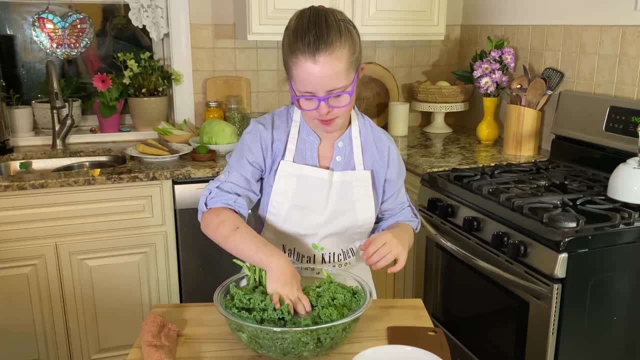 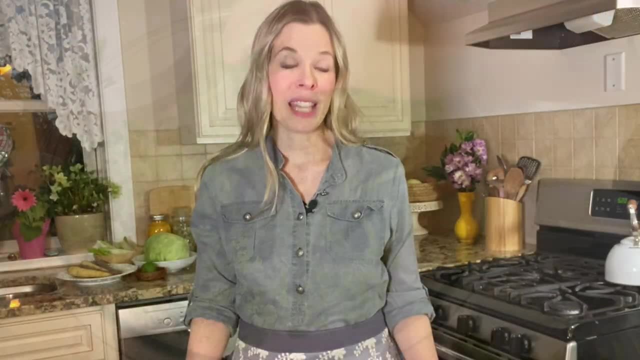 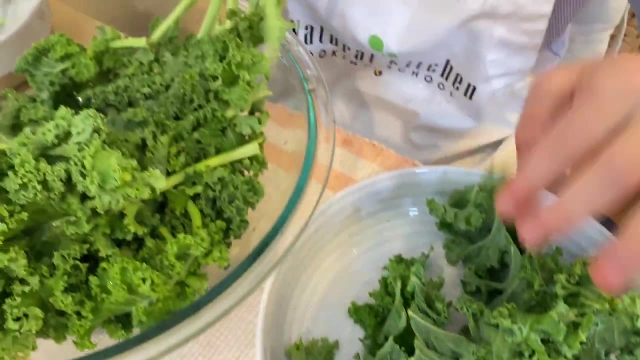 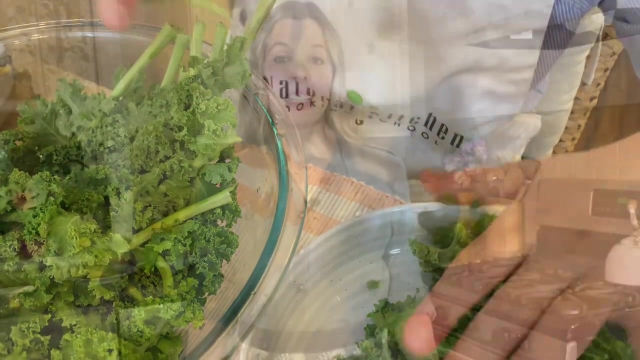 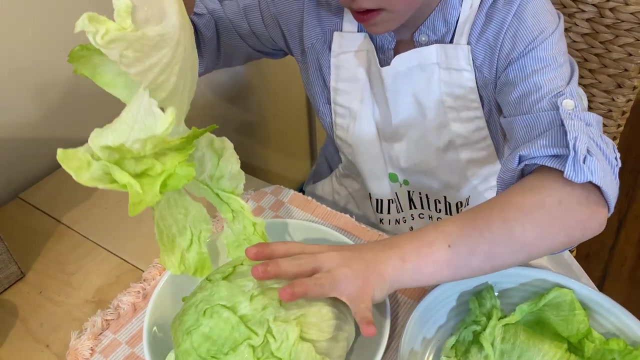 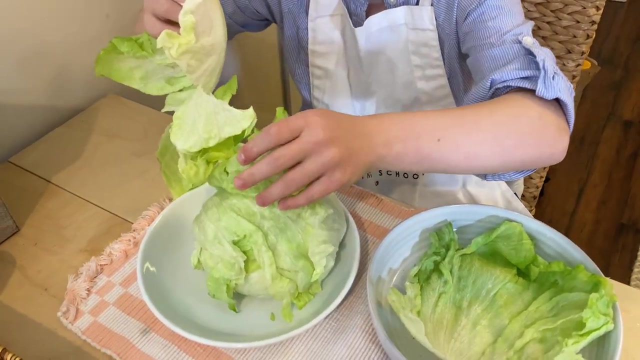 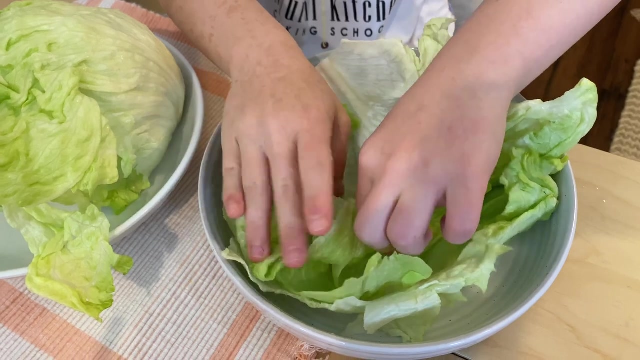 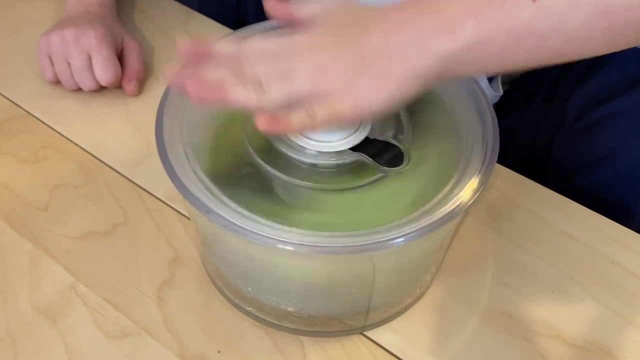 good for beginner chefs include washing fruits and veggies- I like this one- And a pastry scraper. I like this one And a pastry scraper. Pulling kale leaves off the stems, Separating lettuce leaves Using a salad spinner. Juicing citrus like lemons and limes. 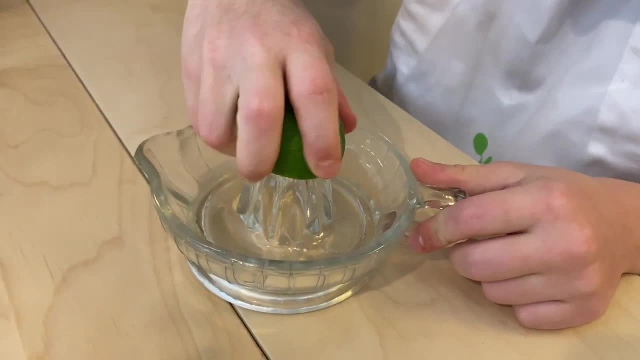 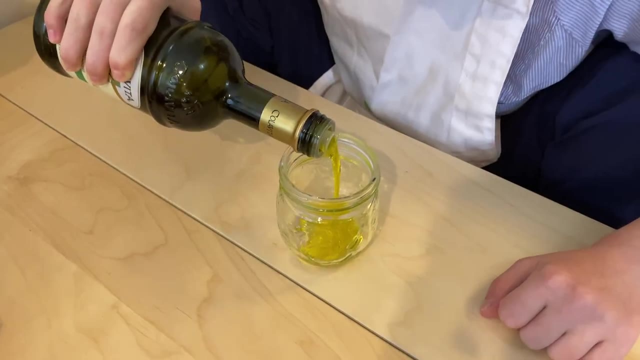 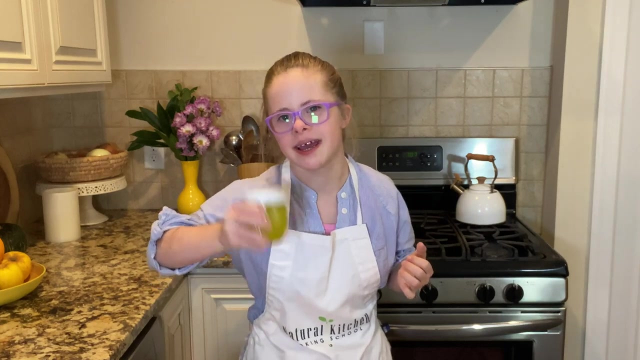 And oranges Helping to measure out the ingredients for a salad dressing in a shaker jar. Pull it, Shake, shake, shake You. okay, Carefully, peeling carrots with supervision, Go ahead. Okay, Hold it down, Hold it down. 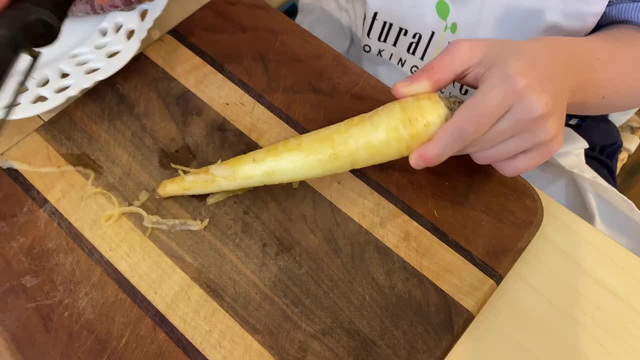 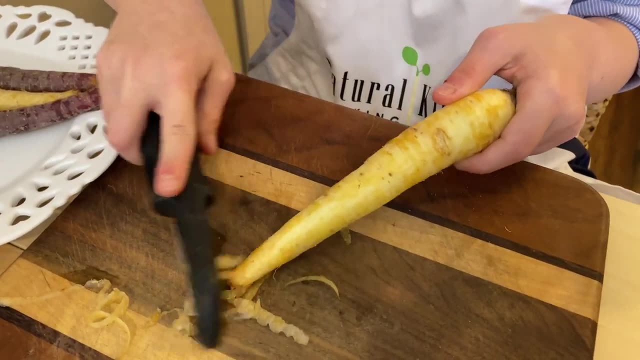 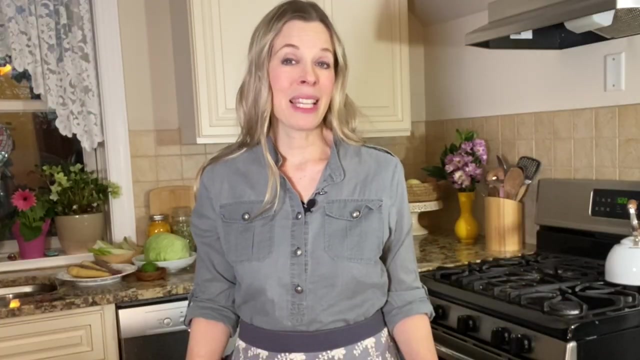 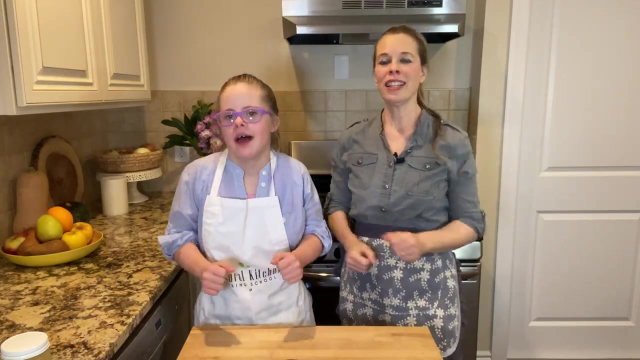 And now peel, Keep turning. Okay, Okay, Okay, Okay, Okay. And of course, measuring, mixing and stirring. All kids love that right. Tip number five is to make it fun. Take stretch breaks when needed. Got our hands. 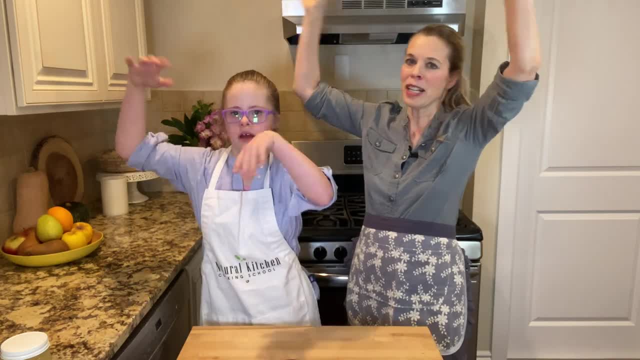 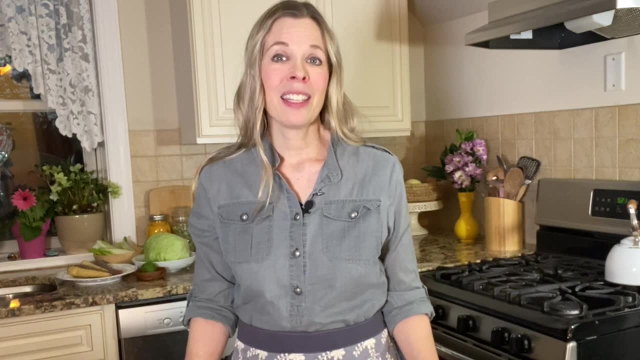 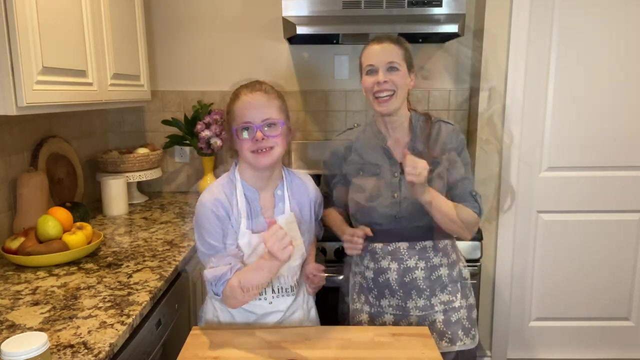 Take our hands, Shake them off. Shake them off A little stretch break, Keep a sense of humor. Keep a sense of humor sensory aspect of food and cooking. You can even do a little kitchen dancing in between cooking. So there you have it, our top five tips to help kids with special 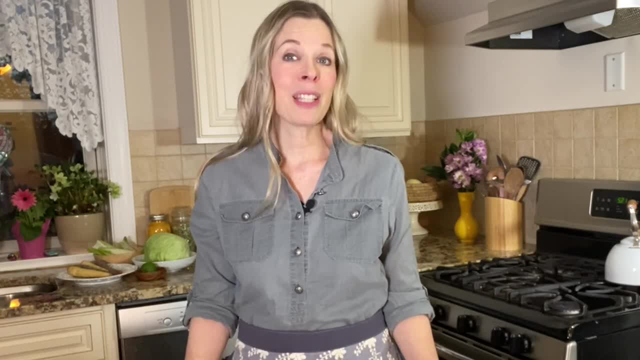 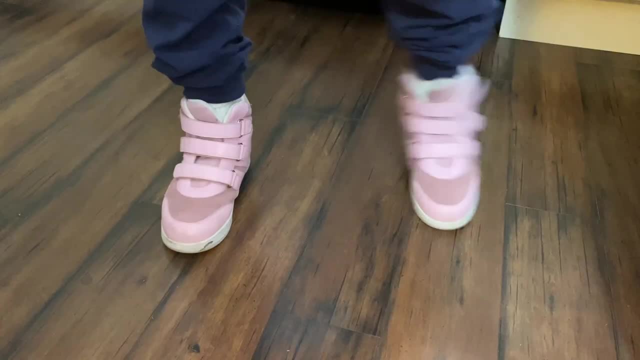 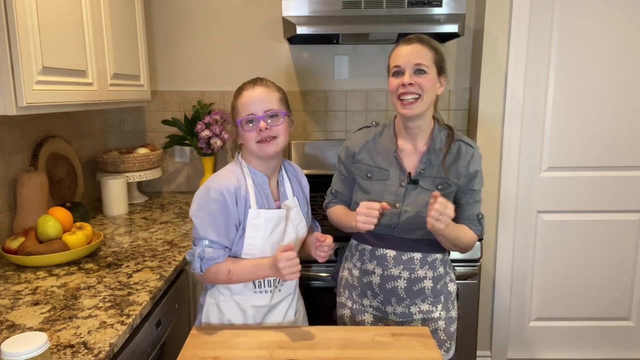 needs. enjoy cooking. Comment below what your favorite tip was, and be sure to like and subscribe for more cooking videos. Thanks for watching. see you in the next video. Bye you.